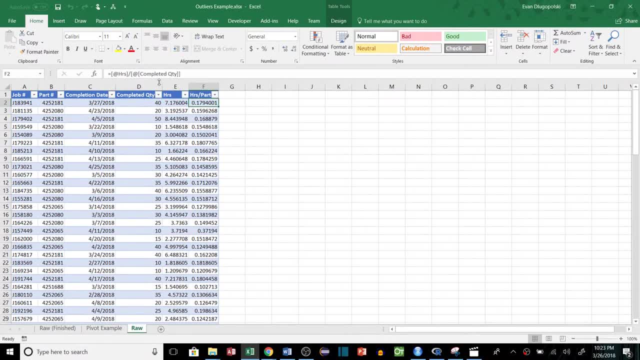 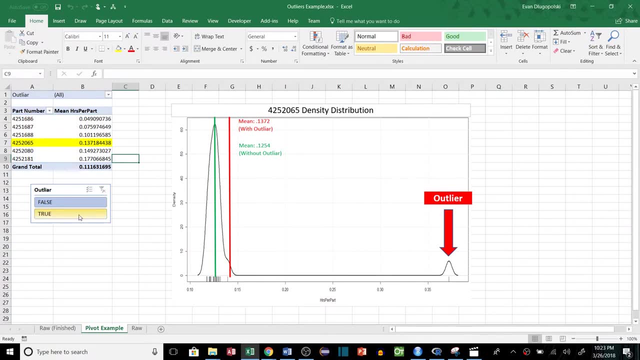 just divide that out to see how long per part it took for that particular raw data to actually make a pivot table. from that to find the mean And just as an example- and I'll go through this step by step afterwards- but we can see that the 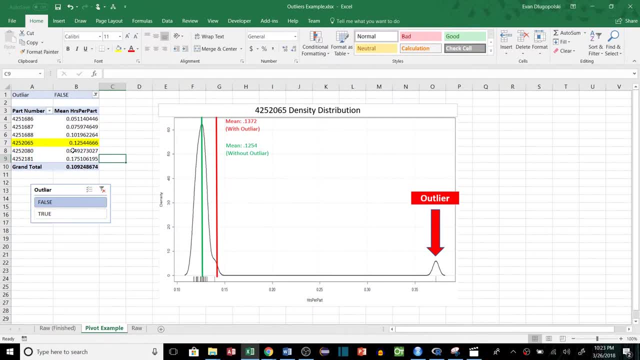 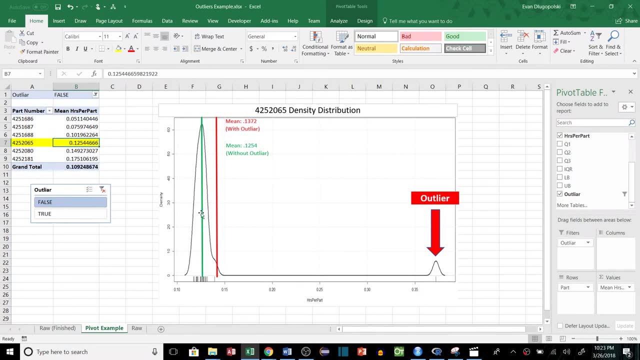 outliers. if I take out the outliers- so I just removed the outlier values- our average for this particular part number drops down to 0.125 hours per part, which is this green line here And that's a more accurate representation of the 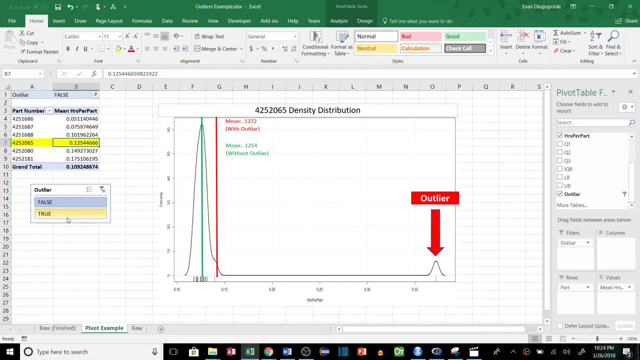 average amount of time that it takes to complete a part, versus if I add this one here or the mean value jumps back up to 0.137, which is actually over here And you can see just visually when we look at the density distribution that that 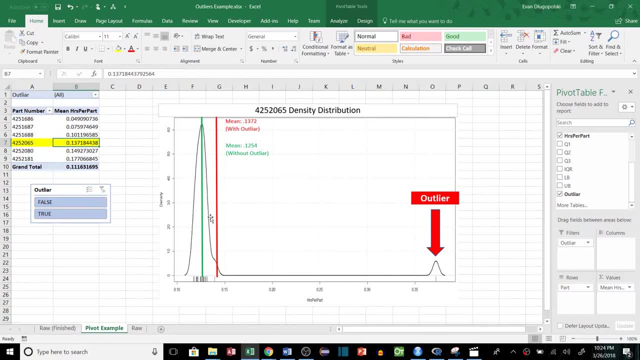 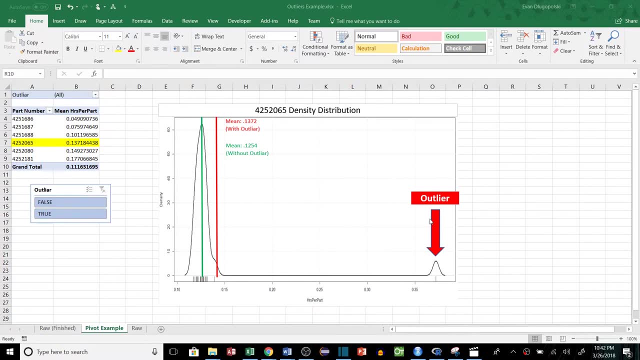 mean value is actually incorrect because this outlier is skewing the average. Quick side note about outliers: I'm not advocating or saying that outliers should always be removed. Outliers often tell us a lot about the data we're analyzing, but in some cases it's necessary and actually more accurate to 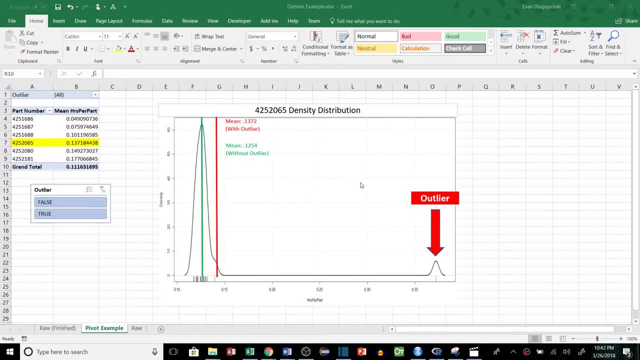 remove them, especially in cases like this, where extreme values are more likely due to human error than not. The method we're going to use for finding our outliers will be the method we're going to use for finding our outliers will be. the method we're going to use for finding our outliers will be. 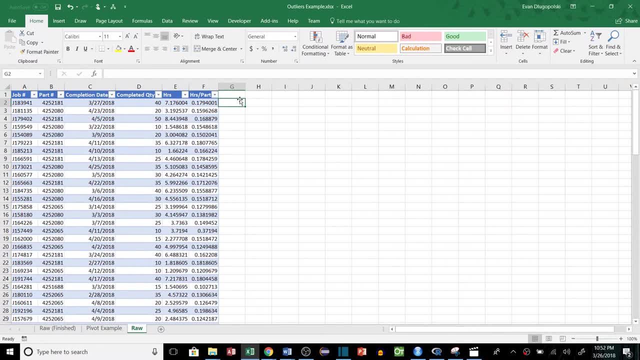 using different quantiles and the interquartile range. So if you've ever made like a box and whisker plot, you're probably familiar with this. but in order to do it we kind of have to trick Excel a little bit or use some special 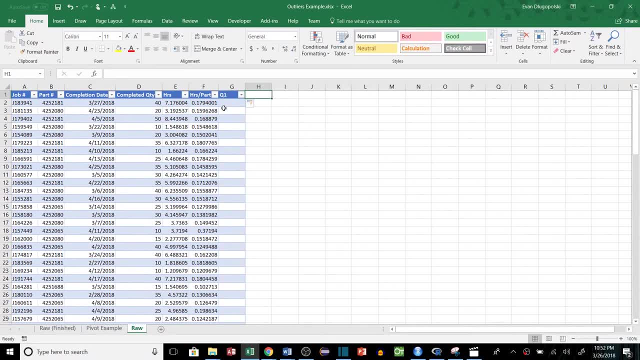 functions. So let's just go ahead and add some columns here for our different quartiles. So we're gonna add q1,, q2, and q3.. And Excel has some functions built in called quantile and we'll use the inclusive And this is gonna be an array. 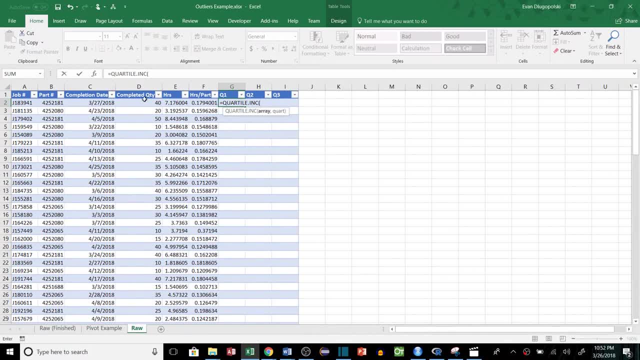 function. so if you're not familiar with quantiles, you're probably familiar with quantiles, you're probably familiar with that. I'll try to break this down And we're gonna say: if our part range- so all of our part values, equals the specific part, 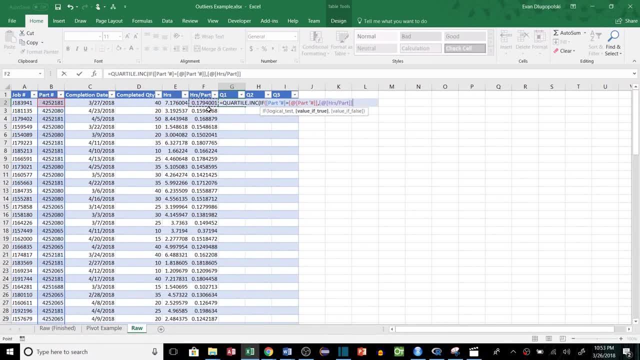 number. then we will feed the hours per part value back into the quartile function And we don't need a value there. and then we need to tell it what quartile we're gonna be solving. So we have to use control and shift and hit enter. 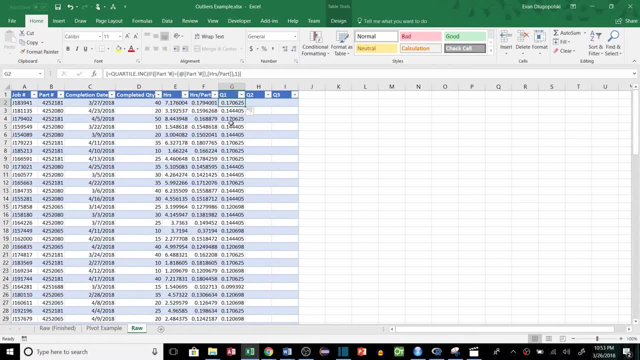 So hold control and shift, hit enter for an array function And that should be our quartile1 value, And then we can just take this and copy it over to here and change this to quartile2.. By the way, that's the same as the median value And 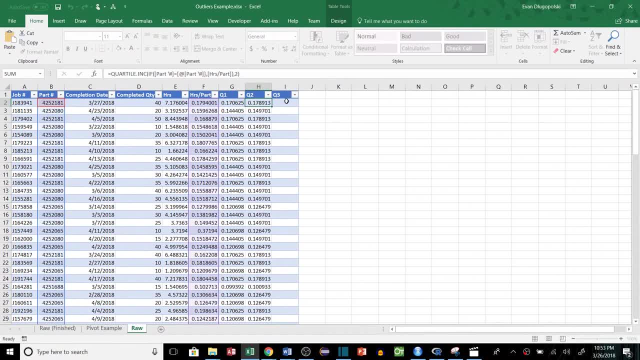 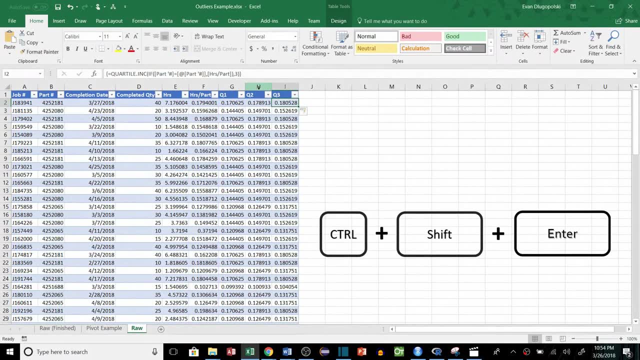 then for a quartile3, it would be the same thing again. Paste that over, Change it to 3 for the third quartile and then control, shift, enter for that. So just to kind of break this down, we use the quartile1 value and then we can change this to quartile2 value. So just to kind of break this down, we use the. 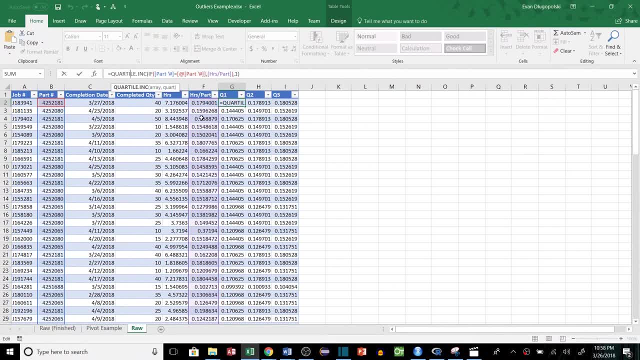 quartile inclusive function, which means that it includes the values that are at the line of each quartile. kind of hard to explain. do a quick google search if you need more information on that. and then the reason we did this array function is we're actually aggregating the data for each part. 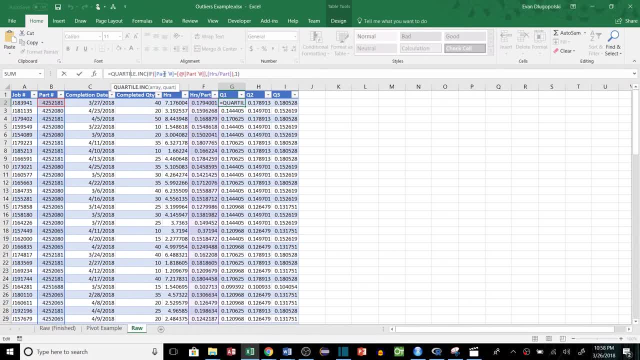 number right here in our table. so what we did is we said: look at each of the part numbers or look at all the part numbers and if that matches the specific row or the part number in this specific row, then we're going to feed all the values, where that matches, back into the quartile function. 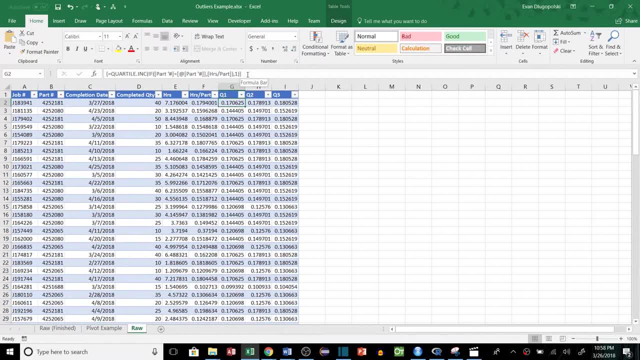 so when we hit ctrl, shift, enter, notice that it adds these brackets so that we know it's an array function. all right, it's all downhill from here. so once we have our quartiles, we can calculate the interquartile range, and that's just simply the third quartile value minus the first quartile. 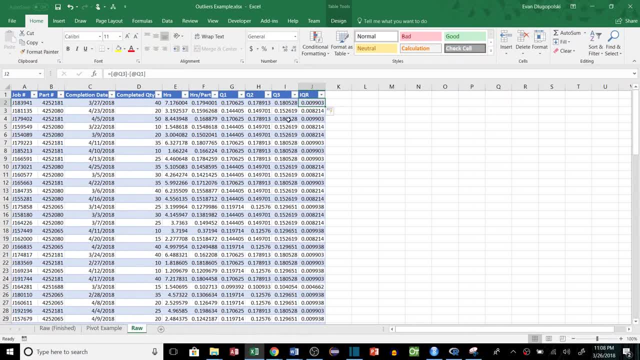 value and that gives us the range between those two quartiles. and then, in order to find our outliers, we need to determine the upper and lower bounds. so let's go lower bound- lb for lower bound and ub for upper bound. so the lower bound is going to be quartile one minus 1.5 times the interquartile range. 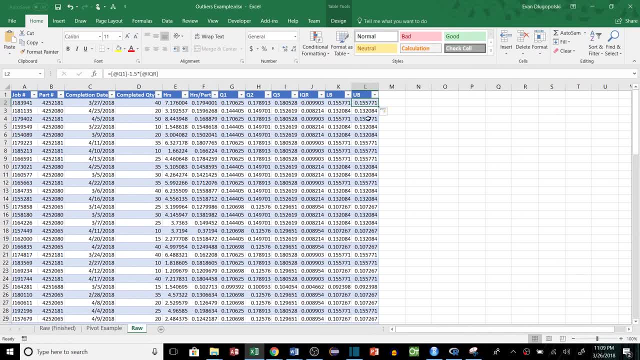 and then we can just copy that over and we'll go switch that to plus and switch this to quartile three for our upper bound. and now that we have our bounds determined, we just need to go ahead and hit ctrl, shift, enter. notice that it adds these brackets. 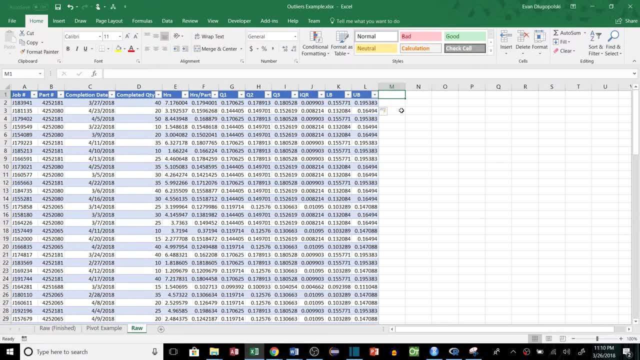 we'll just need to write an if statement to determine if the values are outside of those bounds. so we'll just add a column for outlier and then we'll say if our hours per part value is less than or equal to our lower bound. and we'll have to make this or as well, because we 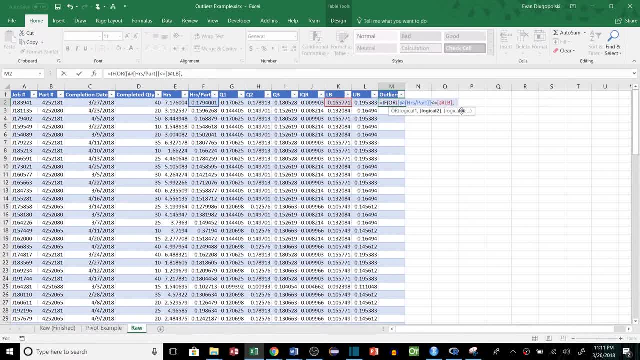 need to do both bounds. so if it's less than or equal to the lower bound, or this value is greater than or equal to the lower bound, and we'll just write an if statement to determine if the values are outside of those bounds, than or equal to the upper bound, close off the or value of true, we'll say it. 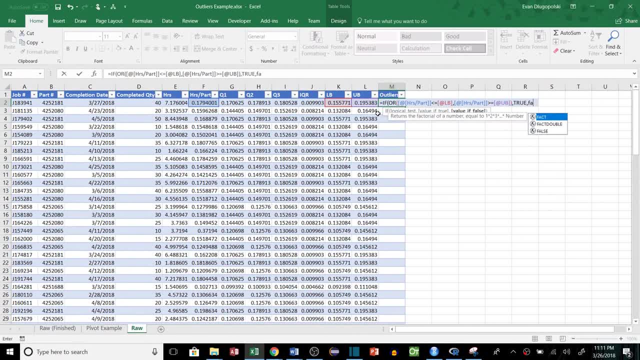 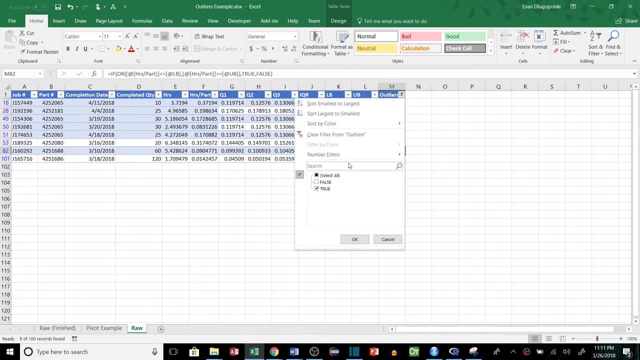 true, it is an outlier, and if not, we'll say false, it is not an outlier. so if we just filter that real quick, we'll see that there aren't too many outliers, but there are a few and, as we saw before, that is enough to skew our data. so if we 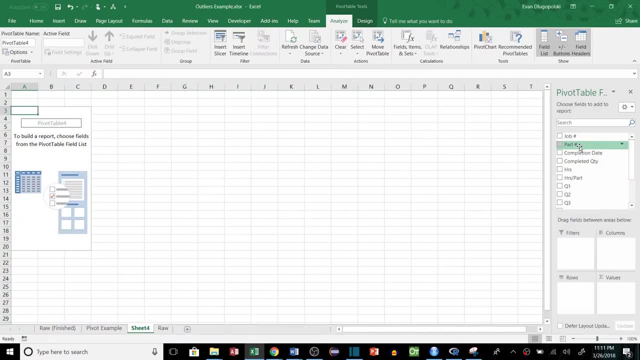 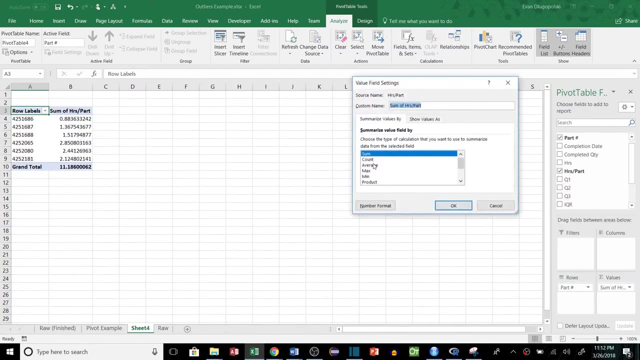 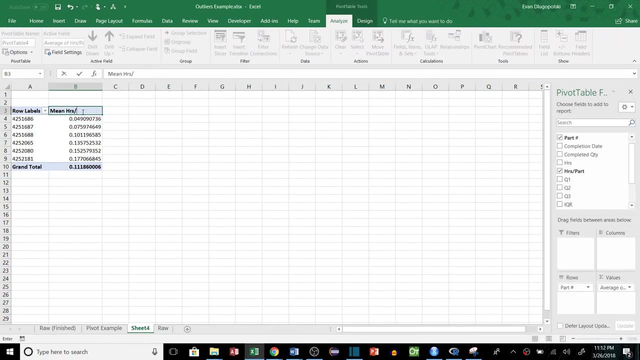 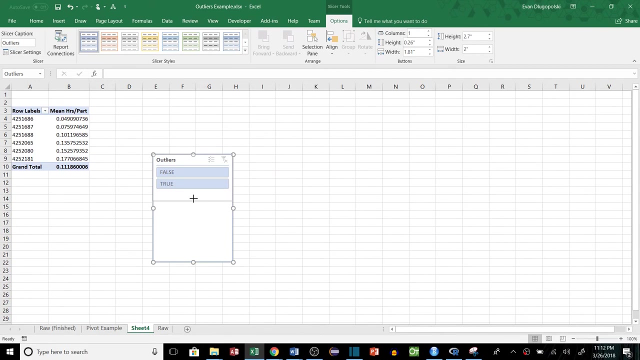 select our data and insert a pivot table and then group by the part number and take our hours per part as a value, select average from our values and this will give us the mean mean hours per part. and if we insert a slicer and select outliers there, now we can actually filter this to either include or exclude. 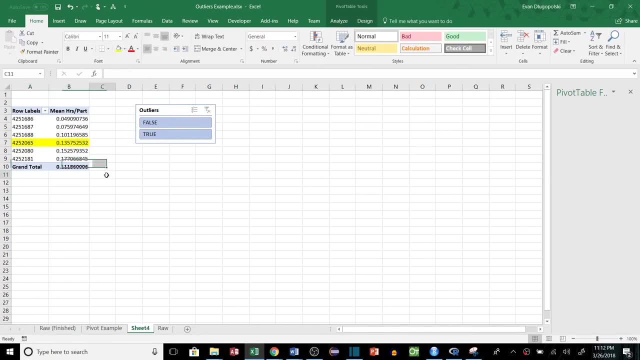 outliers. so we can see a few of the values are affected by outliers. this one in particular is pretty significant. the other ones aren't too significant. this is the. this is the worst one. so that is how you remove outliers from aggregated data and pivot tables. all right, I hope you all enjoyed that one to get more videos, as they